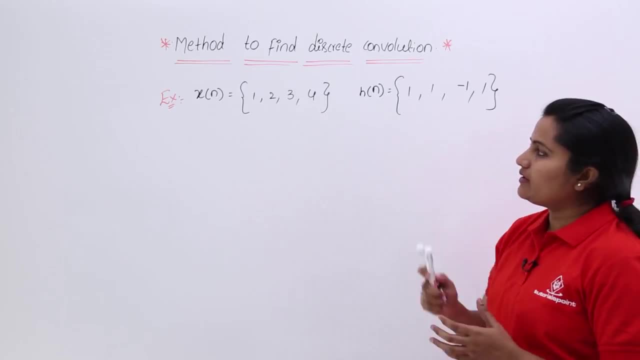 So we are going to discuss the method. So x of n is equivalent to 1,, 2,, 3,, 4.. So that is having 4 samples. and here h of n is equivalent to 1, 1, minus 1, 1.. This is also having 4 samples. 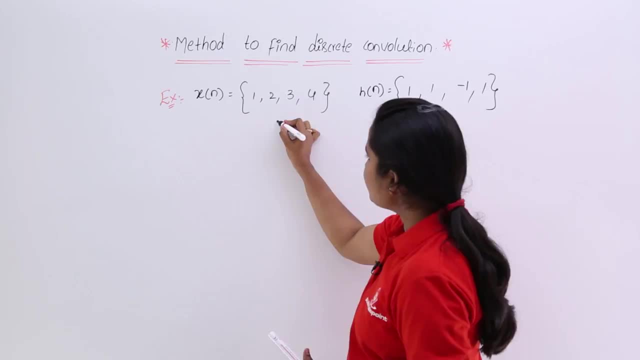 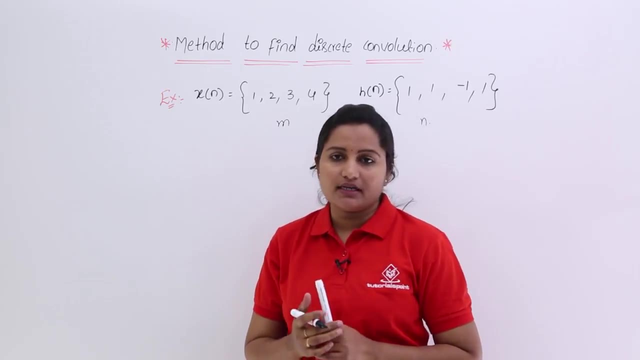 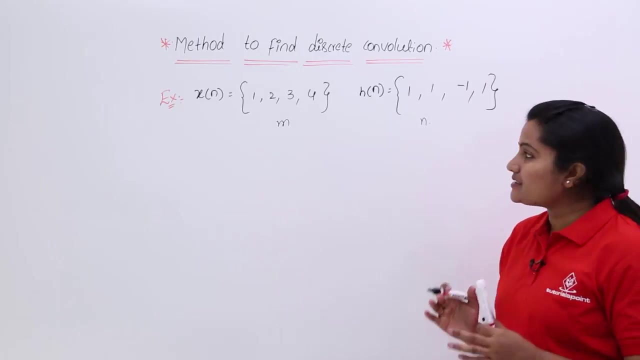 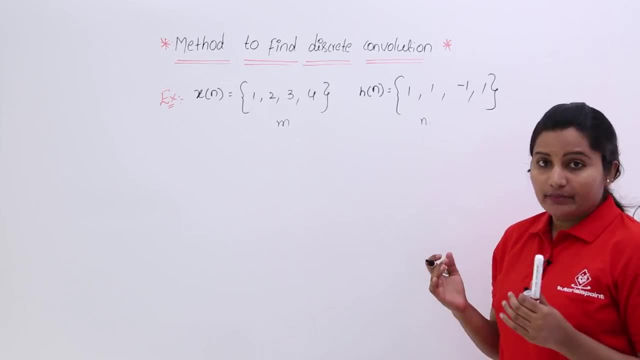 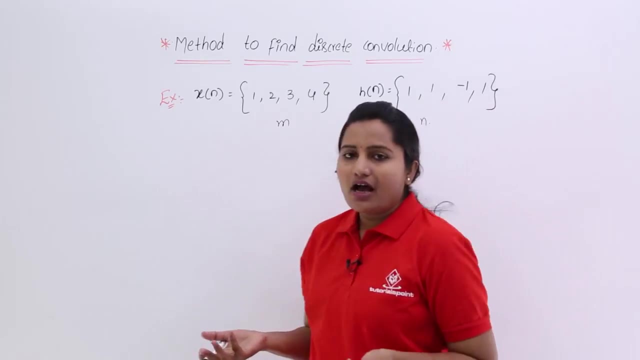 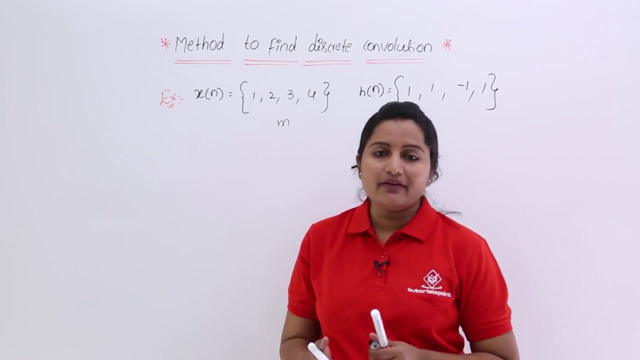 1 samples means 4 plus 4 minus 1 samples. That means 8 minus 1, 7 samples. you are going to get by the end of convolution process. Now, generally, how we can take discrete convolution means you are having a formula at the starting of convolution topic when 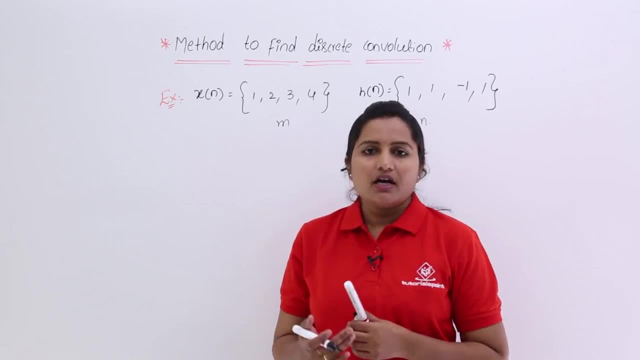 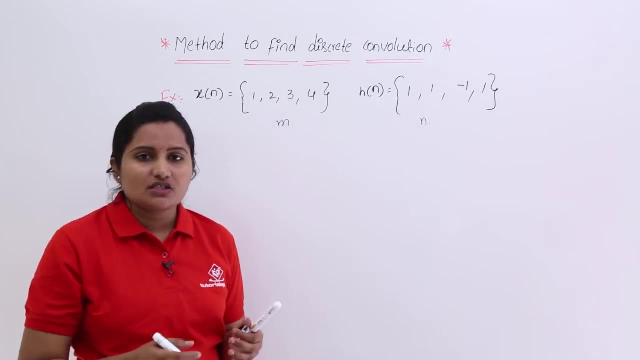 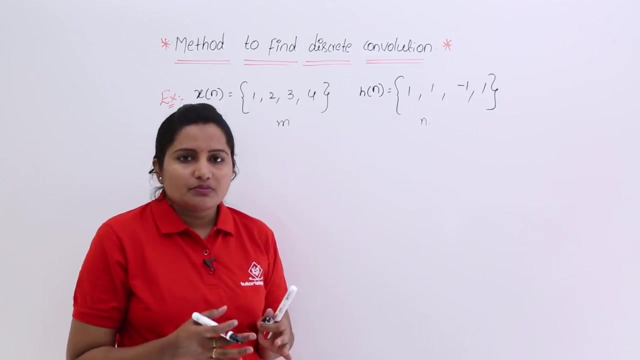 I give an introduction of convolution there itself. I give an discrete convolution idea about discrete convolution. If you consider that formula, each time you need to consider x of n sample and shifted sample of this and like that you need to consider. So that is more. 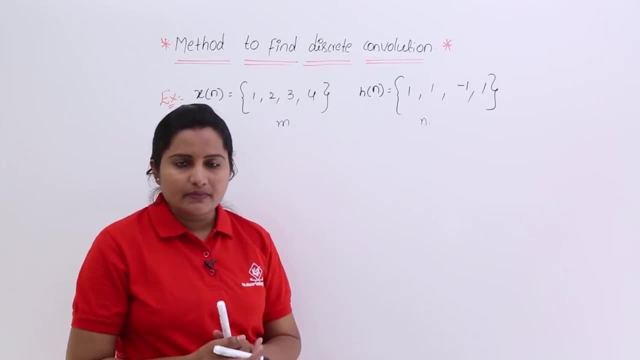 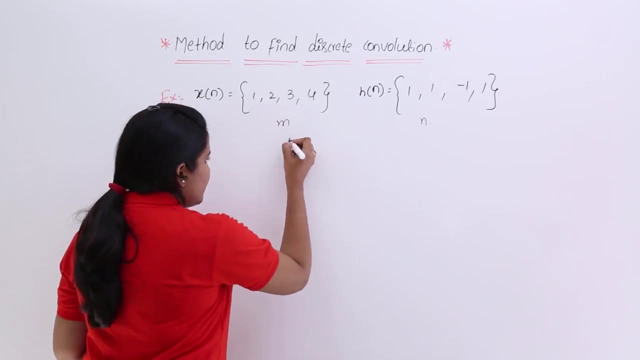 confusing When you are given with this type of samples or discrete convolution. there is a simple way that is called as add and shift method. So here you need to consider like this. So you need to consider like this and you need to write your first signal here. 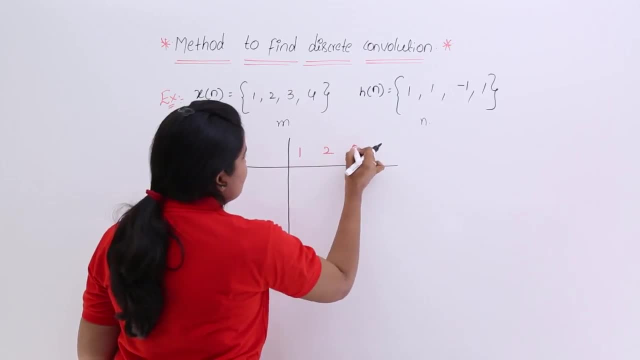 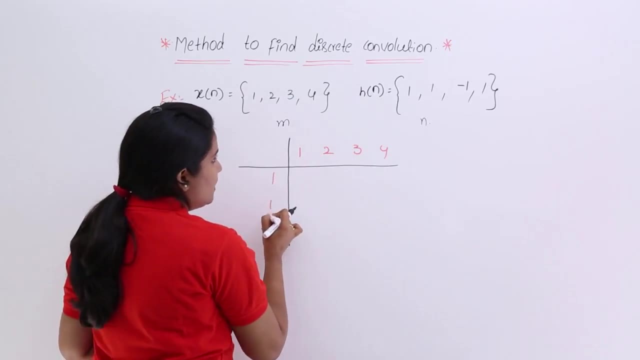 That means I am writing 1,, 2,, 3, 4 here and then, And then I am writing my second signal here. So 1, 1 minus 1, 1, like this, I am writing my second signal. Now what we need to do is we need to multiply crosswise And we 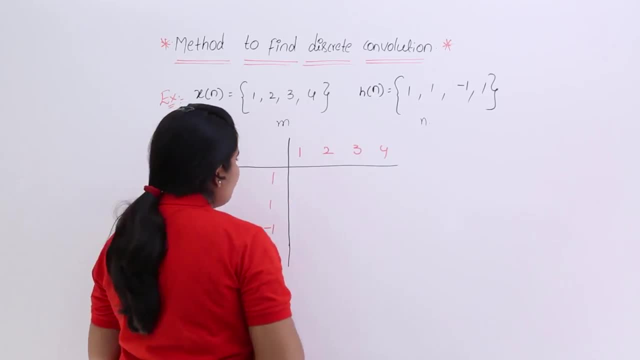 need to write the result in the appropriate set. So here I am just multiplying 1 into 1,, 1, 1 into 2, 2, 1 into 3,, 3, 1 into 4, 4. after that here also 1,, 2,, 3,, 4 after multiplying: 1. we are terminating everything we are going to get maxed out. One is x, 1 is its half. that means 1 is union of 2 and 2 is its half. So you mine, worstified as daily of take fade. 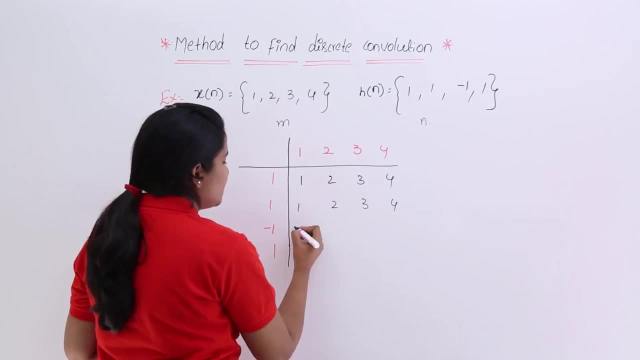 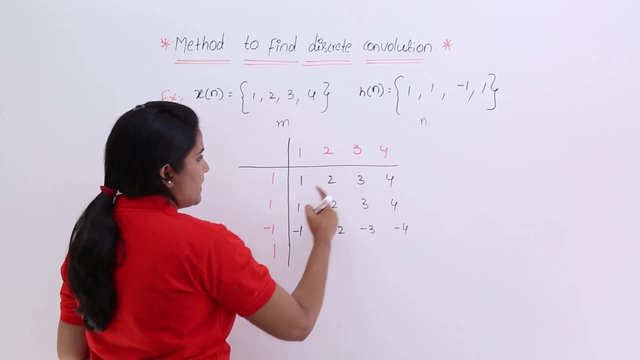 get 1, 2, 3, 4 if you multiply minus 1 with this everything, so you are going to get minus sign for each and every sample. minus 3 minus 4. that means minus 4 into minus 1, into 4 minus 4, like. 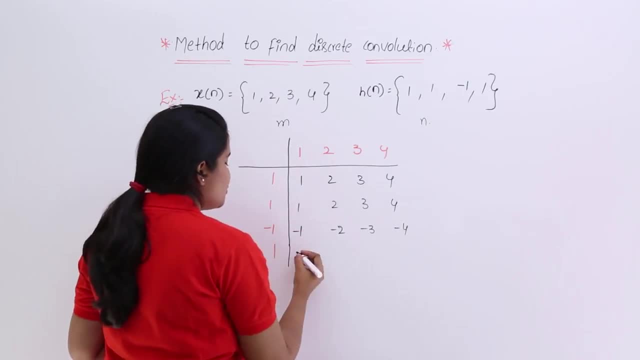 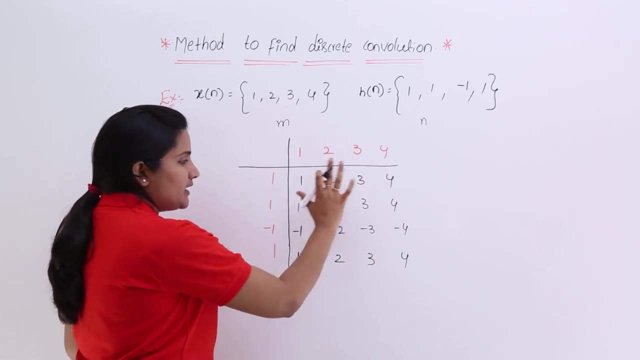 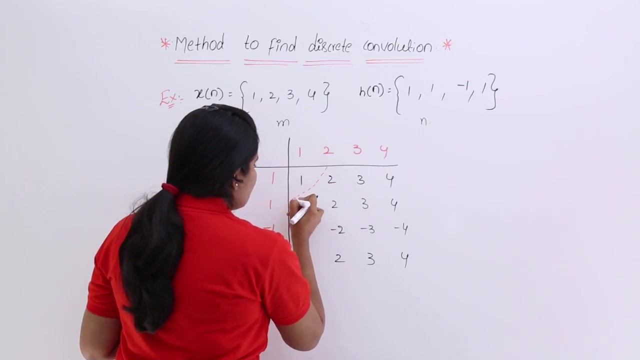 that again, I am multiplying with 1, so I am going to get 1 into 1, 1 into 2, 1 into 3, so 1 into 4. like this: after getting multiplication result, like this, you need to draw vertical lines. you need to draw diagonal lines like this. so, like this, you need to draw diagonals. 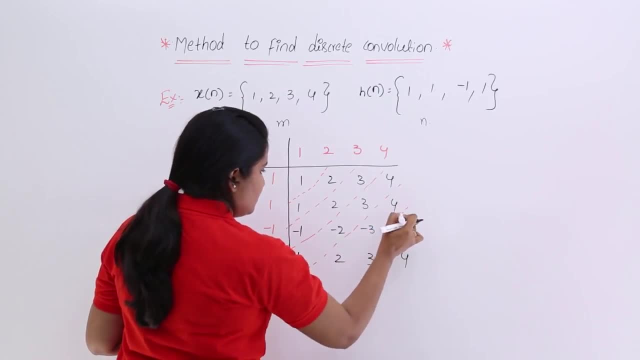 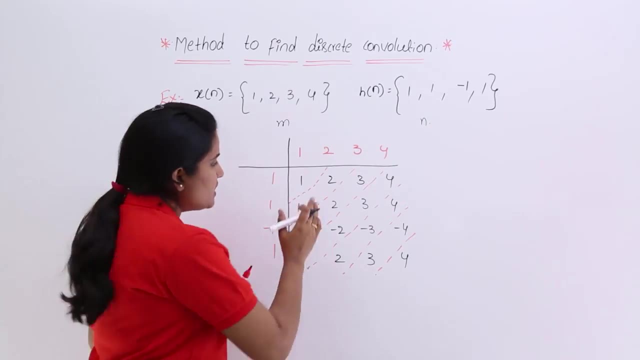 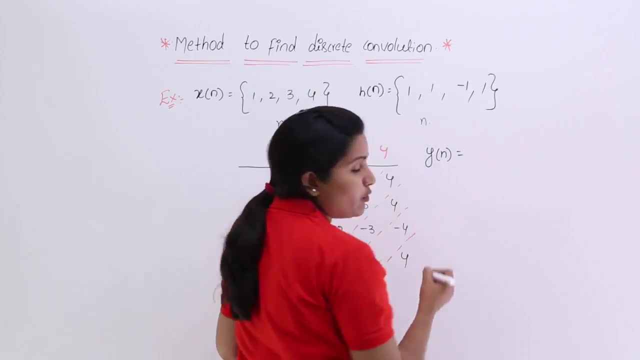 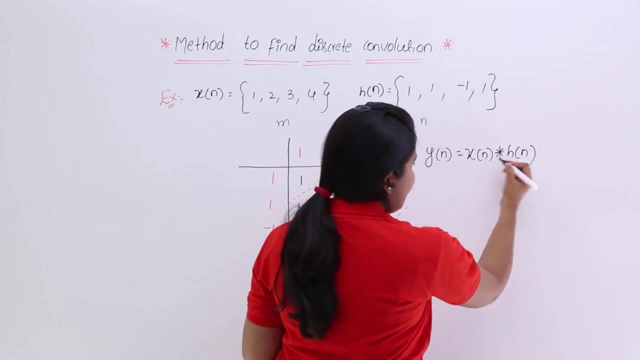 so now you need to draw diagonal like this. so here what you need to do is so in this diagonal, only one sign is there that you need to consider your first sample of your response, which is the convolution of x of n and h of n. if y of n is the convolution of these two, then y of n is equivalent to this 1. 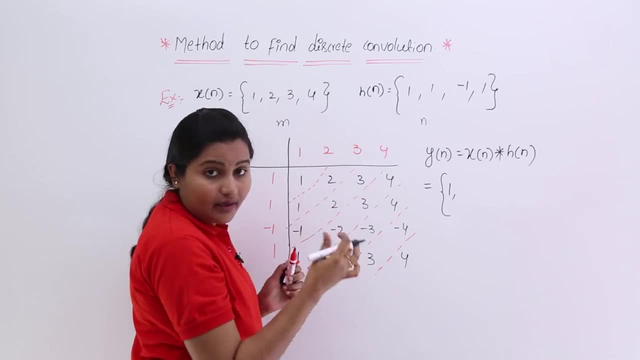 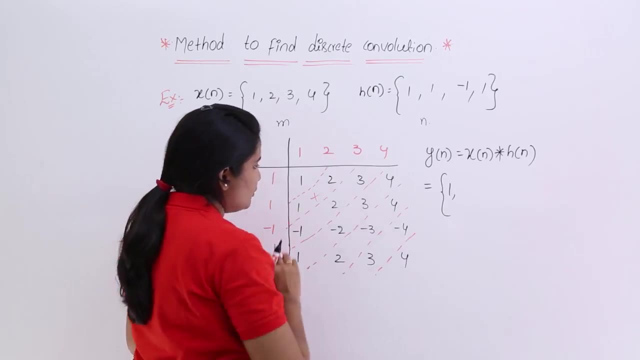 comma. second sample can be obtained from this second diagonal line. that means 1 plus 2. you need to consider 1 plus 2. you need to consider if you consider 1 plus 2, you are going to get 3 here and if you are, if you are adding these three samples, 3 plus 2, 5 minus 1. so 3 plus 2, 5 plus. 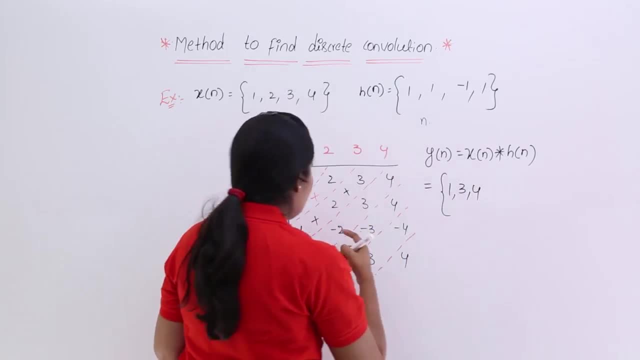 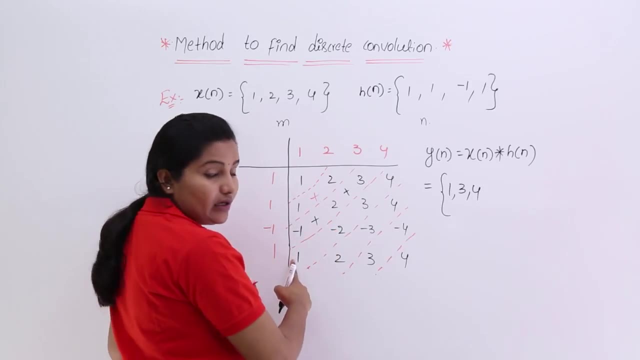 minus 1 means you are going to get 4 here and here, 4 plus 3, 7, 7 minus 2, so 5, 5 plus 1, 6, 6 you are going to get here, and after that you are going to get 3 here and after that you are going to get. 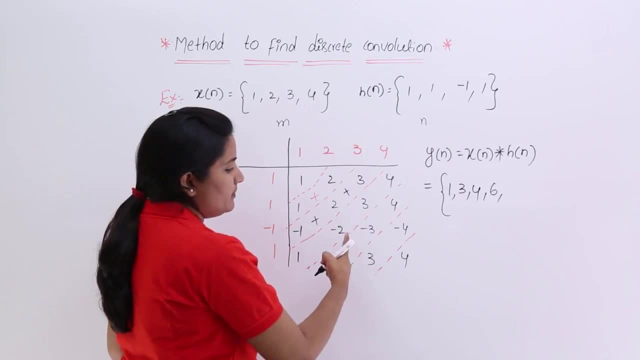 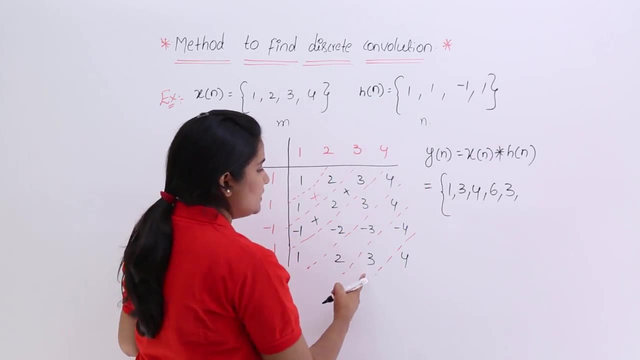 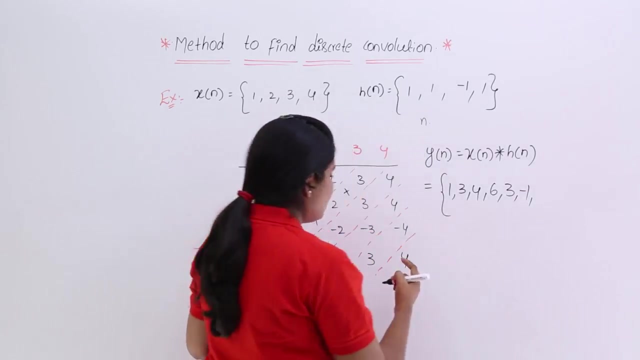 4 minus 3, 1, 1 plus 2, so you are going to get 3. and here you are having another diagonal line: minus 4 plus 3. minus 4 plus 3 means you are going to get minus 1, so comma. finally you are having. 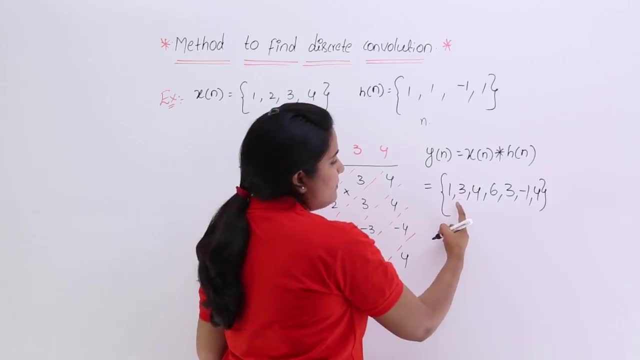 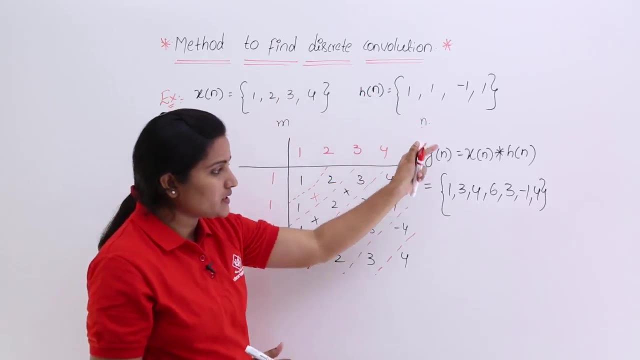 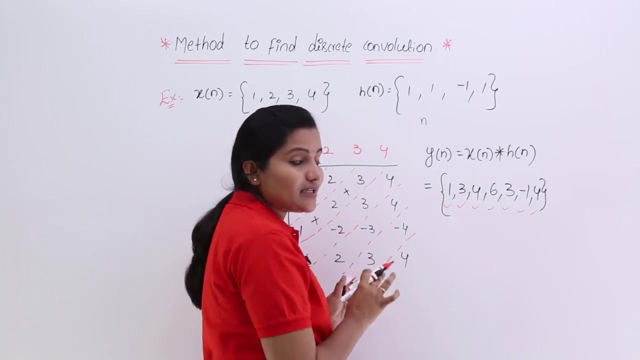 4. here you can observe how many samples you got at the response when you convoluted m samples with n samples or 4 samples with n samples. so you are going to get 4 here and after that you are going to get 4 samples totally. you got 1, 2, 3, 4, 5, 6, 7, 7 samples you got in the response of the. 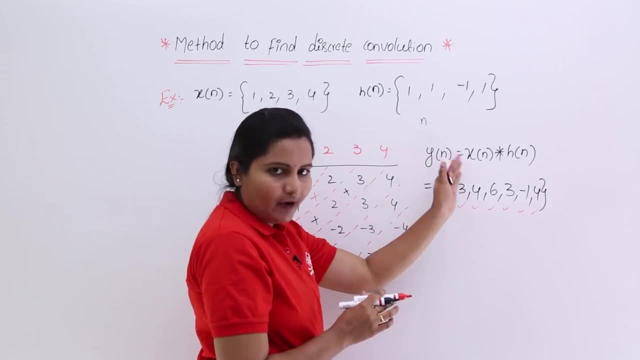 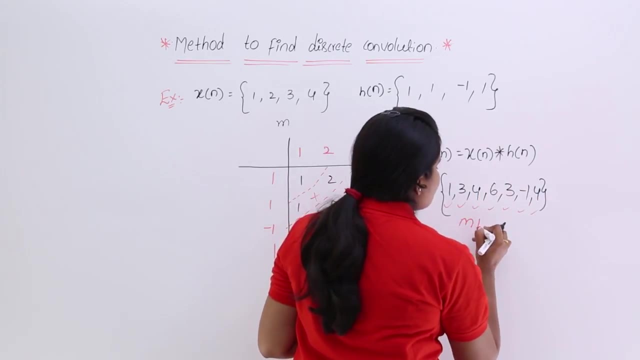 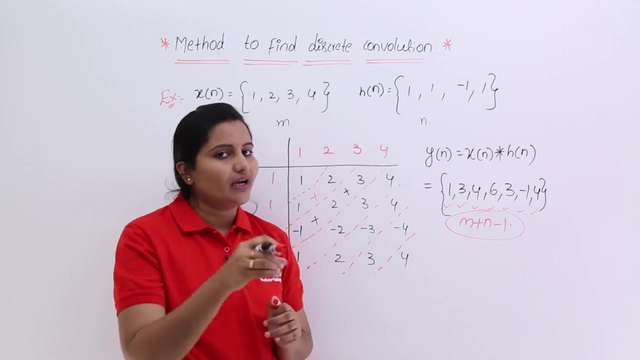 signal or response of the system, or y of n, where it is equivalent to convolution of x of n and h of n. that means you got n plus n minus 1 samples. this is very important point. based on this sample number also, you can trace the option when you convoluted with m samples with 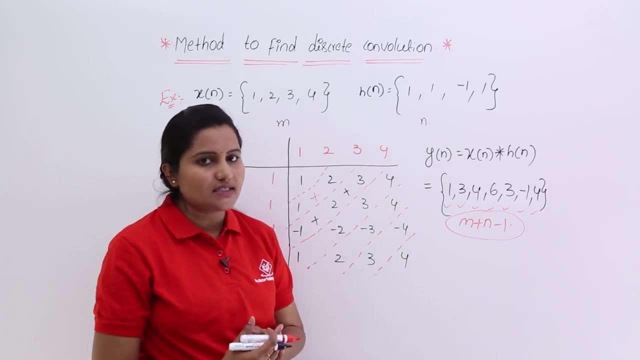 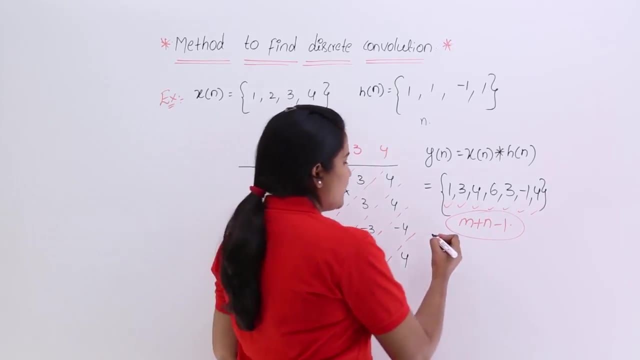 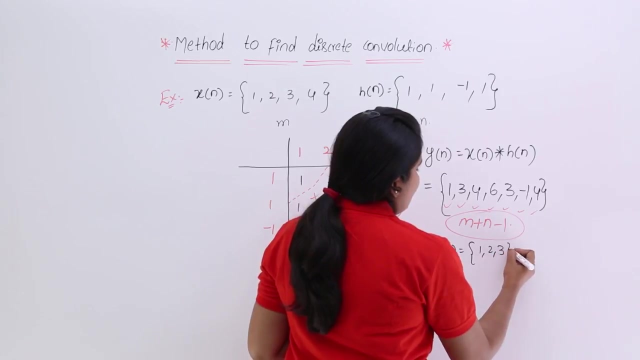 n samples, you are going to get m plus n minus 1 samples. so now, on the same 8 like this, i am going to consider another simple example, that is, for example, x of n is equivalent to some 1, 2, 3, and h of n is equivalent to some 1 and minus. 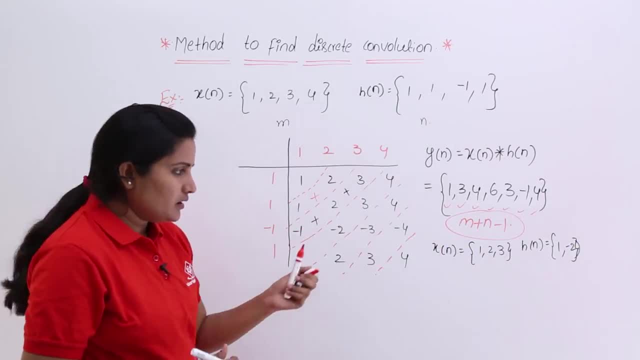 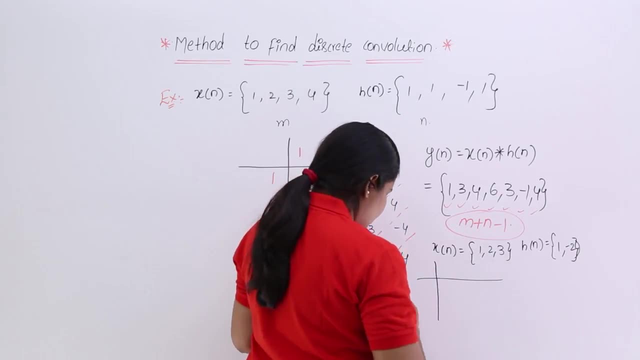 2, so these are the samples that we need to convolute. then i am going to get the samples according to this structure. so on that side- which is that is very important, because for both going to consider again the same procedure, I am going to consider 1, 2, 3 and h of n is 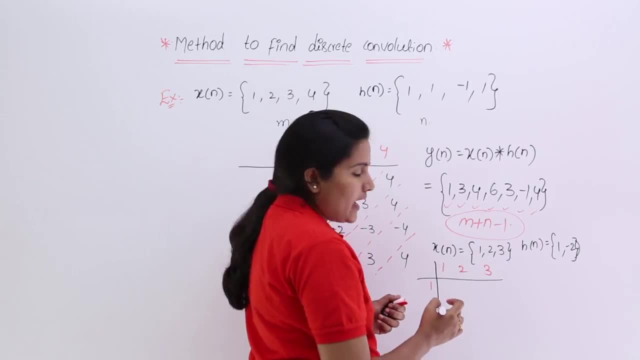 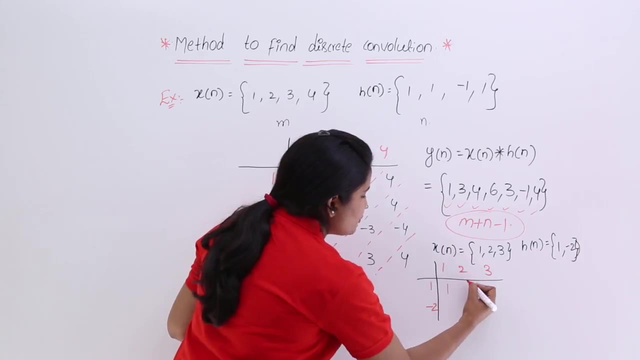 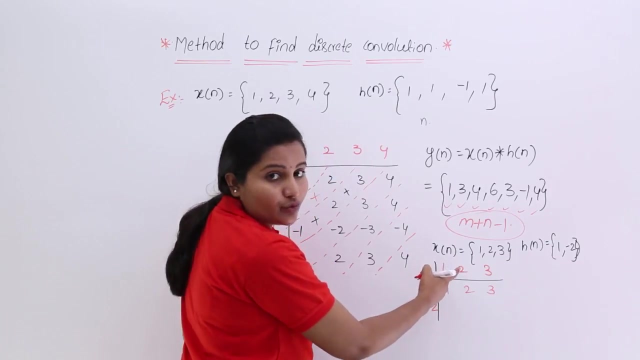 equivalent to 1 minus 2, and here, if you multiplied these two, then how you are going to get 1 into 1, 1, 1 into 2, 2, 1 into 3, 3 and after that, here, if you multiplied minus 2 into 1, here 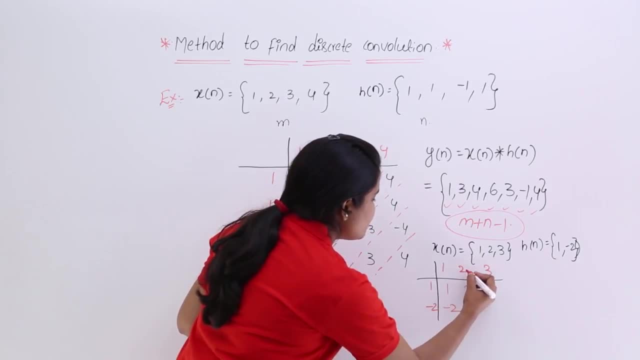 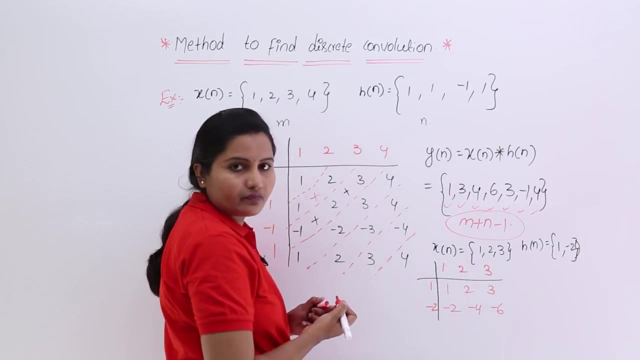 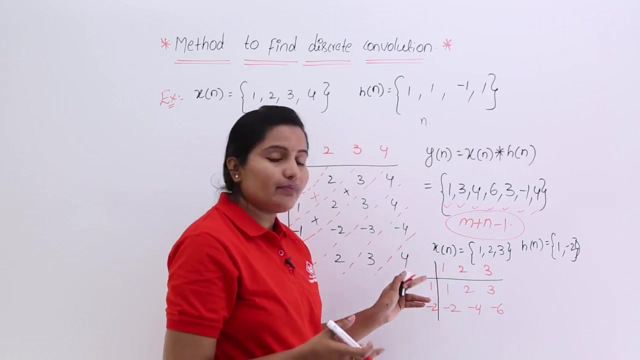 so you are going to get minus 2, minus 2 into 2, minus 4 here, 2 into 3 and minus. so you are going to get 6 here if you consider diagonal. so in this case, how many samples you need to get? you got 3 samples and you are convoluting with 2 samples. so m plus n minus 1 means you.